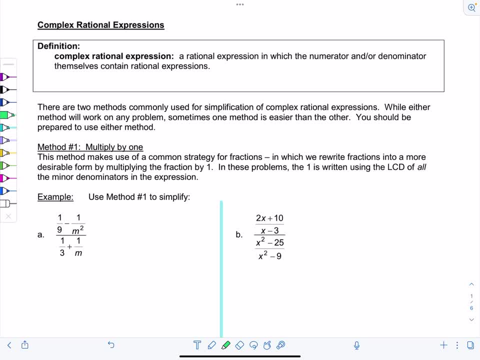 you can use them appropriately in any circumstance. So first method, my favorite one, is when you multiply the entire expression by one. This method makes use of a common strategy for fractions, in which we rewrite fractions into a more desirable form by multiplying the fraction by one, And in these problems, the one is written. 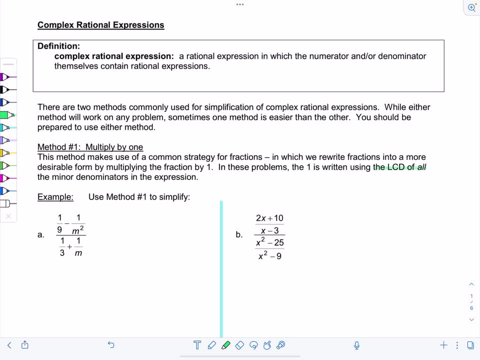 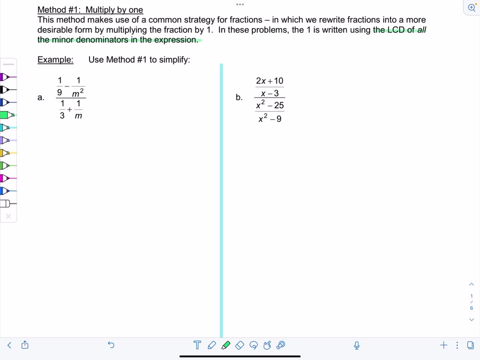 using the LCD or the least common denominator of all the minor denominators in the expression. So what the heck does that mean? I'll show you right now with an example. Use method number one to simplify. Okay, so we have one over nine minus one over m squared. 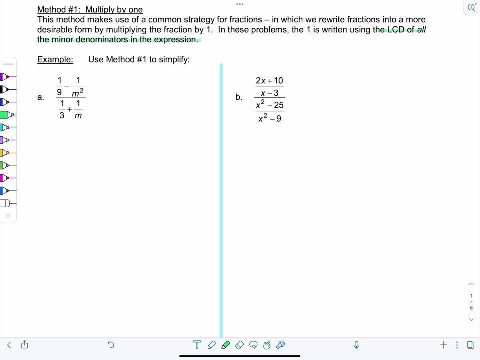 over one over three plus one over m. The minor denominators are the denominators of the fractions within the fraction. So nine is a minor denominator, M squared is a minor denominator, Three is a minor denominator, and so is m. Okay, our job is to figure out what is the LCD. 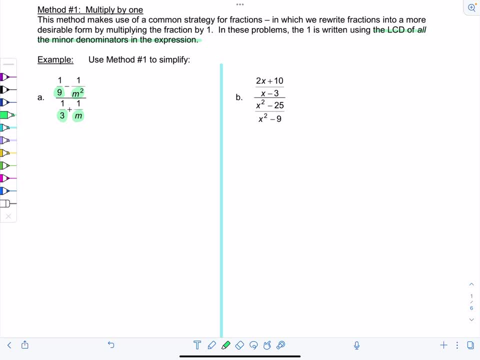 for all four of these denominators. Okay, so pretend like you're gonna add them all together, but that's not what we're gonna do. And notice the LCD is nine m squared. So, since the LCD is nine m squared and we're gonna use method one here, 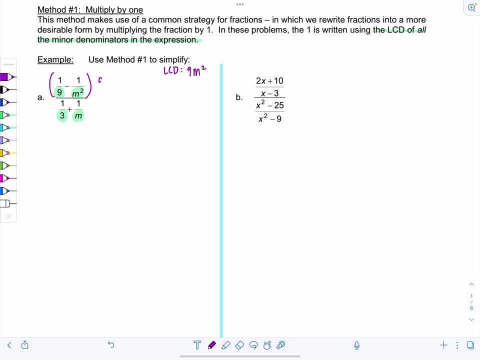 what that means is I'm gonna multiply the numerator by nine m squared and the denominator by nine m squared, And I'm allowed to do this because I'm multiplying by the same thing in the numerator and denominator, so I'm just multiplying the fraction by one. 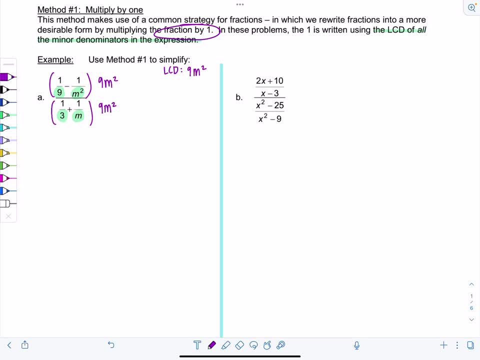 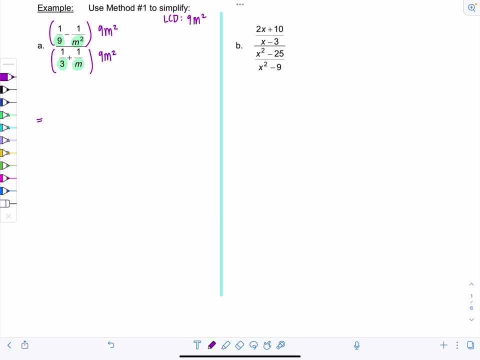 Okay, now this next step. I'm really gonna break it down for you to see how to simplify and multiply. multiply everything by this 9m squared. When you get more comfortable, you can start skipping steps and doing stuff in your head. Okay, so in the numerator we have that 1 over 9 minus 1 over m. 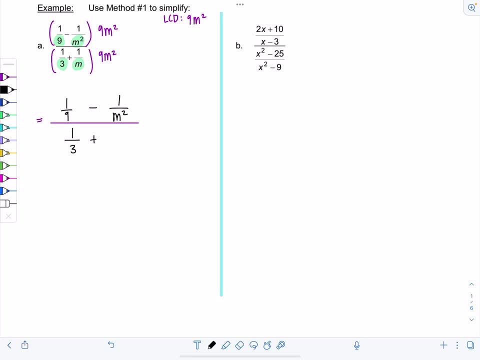 squared, And then in the denominator we have 1 over 3 plus 1 over m, And now I'm multiplying everything by 9m squared, So it distributes to both terms in the numerator. And if you need to remind yourself, go ahead and put that 9m squared over 1, okay, as you distribute. 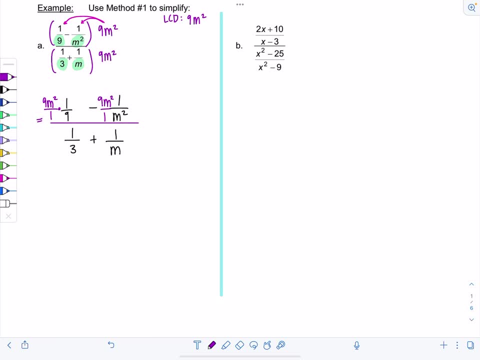 it: 9m squared over 1.. And then it also distributes to the terms in the denominator. So let's write it out here: 9m squared over 1, 9m squared over 1, okay. So let's write it out here: 9m squared over 1, 9m squared over 1, okay. 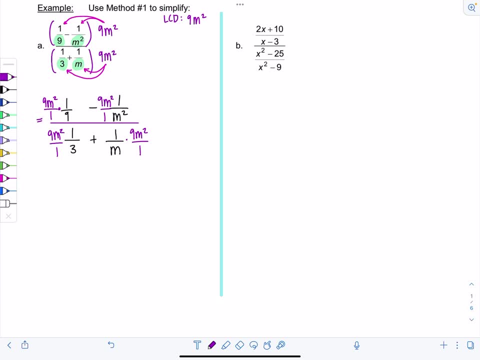 When you multiply the LCD to the numerator and denominator, it's always over 1, over 1, okay, Good, Now let's clean things up. So notice here: in this first term, what can we cancel out? I can cancel out a 9.. So I'm just left with: now m squared okay for that first term. 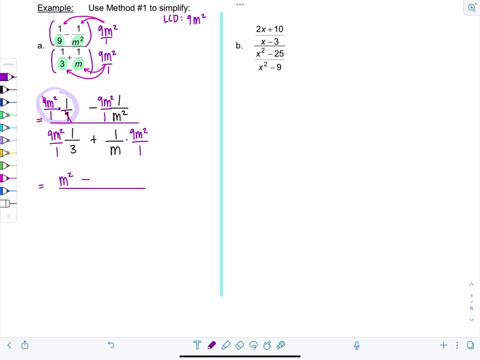 minus. And then now let's look at the second term in the numerator: What's going to cancel out? I can cancel out an m squared right, So I just have a 9 left over, Perfect. Now let's move our attention to the denominator. What can we cancel out here? 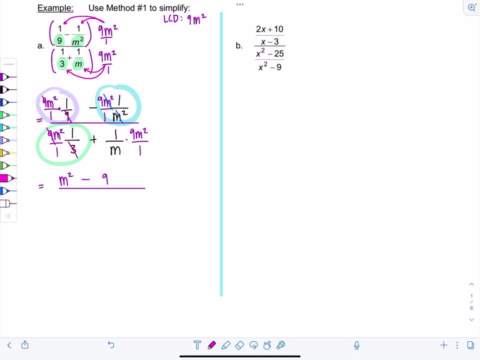 I can cancel out this 3 with the 9 in the numerator. Now it's going to become just a 3.. I still have that m squared though, So we've got 3m squared plus, and then last term down here. what's going to cancel Just that m? 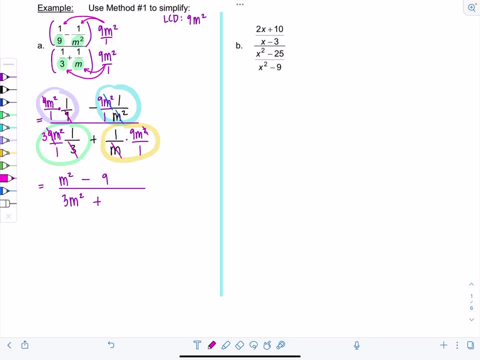 with one of the m's from the numerator, So we have 9m left over. All right, Now here is where you need to check that you've done things correctly. There should be no fractions In the numerator or the denominator anymore. If there still are, then that means either you. 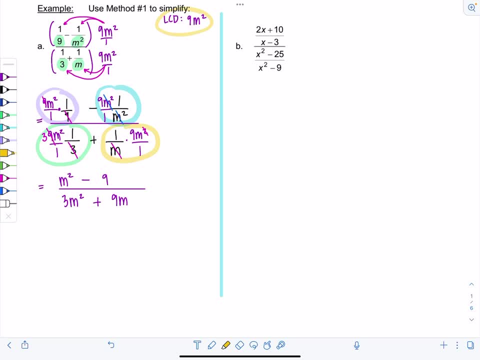 pick the wrong LCD or you didn't distribute and cancel correctly. So at this point, right here, you should be fraction free. Now it's just a matter of cleaning things up, Okay. So, yep, I'm super happy. There's no fractions in the numerator, no fractions in the denominator. 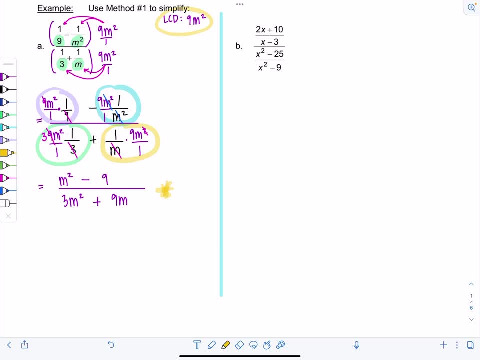 I want to see if I can simplify and cancel. Before you even think about canceling, you've got to factor the numerator and denominator Completely. so look at the numerator m squared minus 9.. Do you recognize that That's a difference of squares? So that will factor into m plus 3. 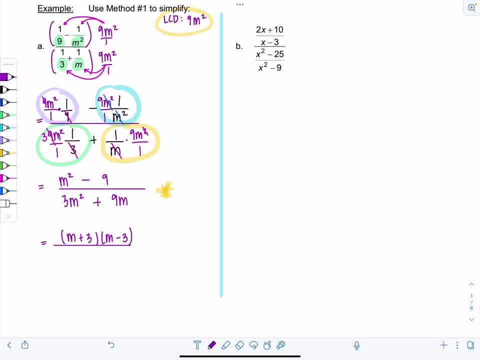 times m minus 3.. All right, very good. And then, looking at the denominator, we have 3m squared plus 9m. There's just two terms. So what can I take out? What's the greatest common factor that I can take out from both those terms? 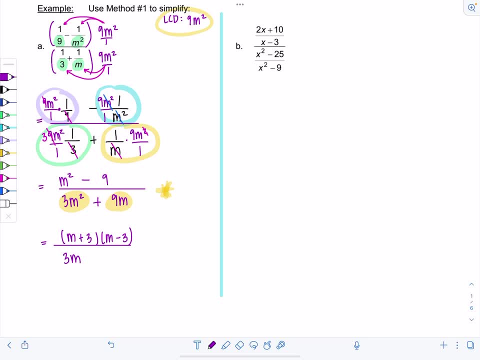 terms. That's right, it's a 3m, So I'm going to take out 3m and now I'm just left with m plus 3.. Lovely, Now I've fully factored the numerator, fully factored the denominator, If I see any. 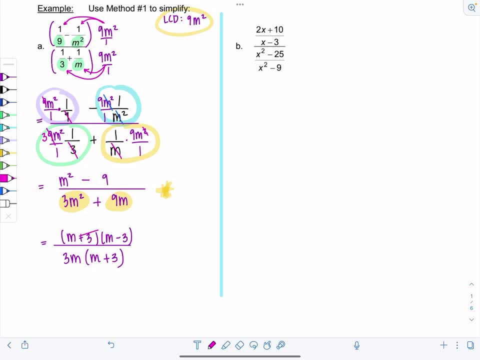 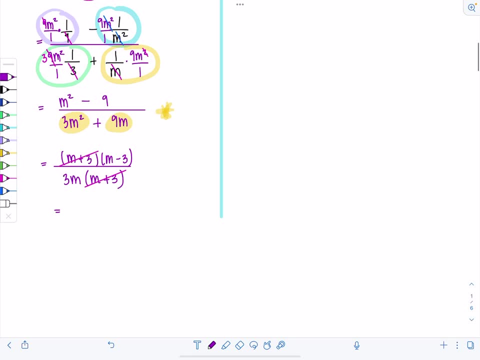 common factors. I can cancel them out, and I sure do. I see m plus 3, so those are going to cancel. And then now final answer: we're left with m minus 3 over 3m. okay, You can't cancel any further. 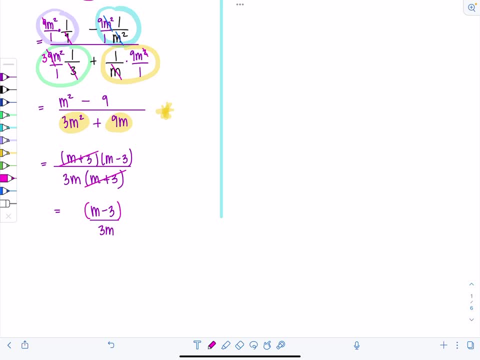 We don't normally put the parentheses around the m minus 3 like that when it's the only factor left over in the numerator. but keep in mind that m minus 3 stays together. It's like a little family. If there was an m minus 3 down here then we could cancel. okay, But you can't do anything. 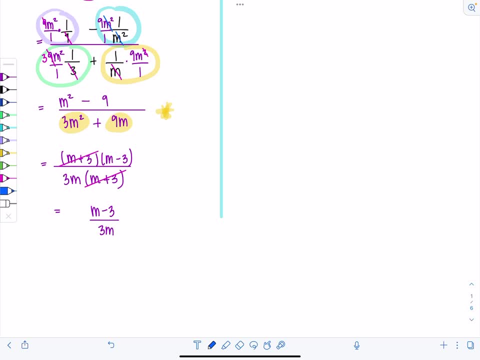 weird, like start canceling these M's. No, no, no, Don't break up the family, Don't be a homewrecker. That's an illegal math maneuver. So there we go. That's our final answer. All right, good, Let's look at another example, a little bit different. 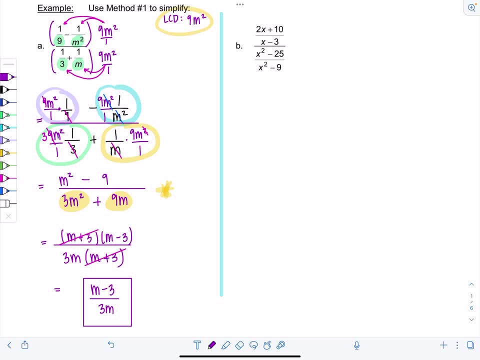 Here we have 2x plus 10 over x minus 3, over x squared minus 25, over x squared minus 9.. Okay, so remember, when we find the LCD, we have to look at the minor denominators. What are the minor denominators? They're the denominators of each of the fractions from the 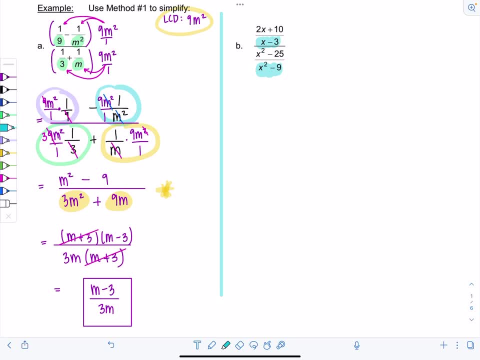 numerator and denominator. And I can't quite find the LCD right now because x squared minus 9 isn't fully factored, So let's go ahead and do that. first. I'm going to rewrite everything. I have, 2x plus 10 over. 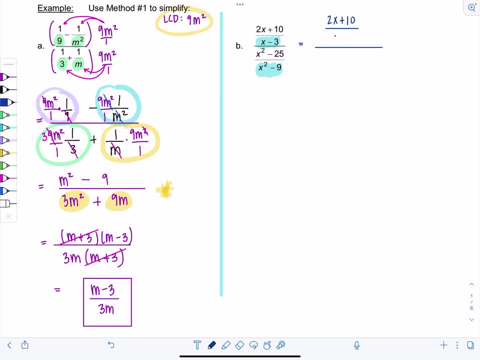 x squared minus 9 over x squared minus 9.. So I have 2x plus 10 over x minus 3.. And then I have x squared minus 25.. I'm just going to factor the denominators for now Over x plus 3 times x minus 3.. So now the minor denominators are here. 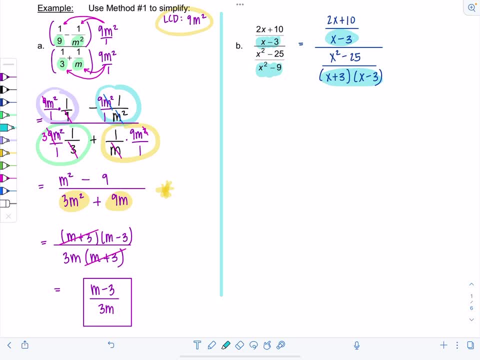 x minus 3, x plus 3 times x minus 3.. And what's the LCD for those two denominators? That's right, It's x squared minus 3 over x plus 3 over x plus 3.. And then I have x squared minus 25.. 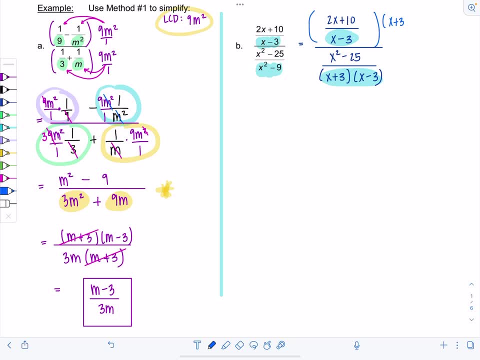 x plus 3 times x minus 3.. So that's what I'm going to multiply by in the numerator and the denominator, And then one more here And, like I said, if you want to remind yourself, each of these is over 1.. Okay, so you know how to cancel appropriately. Go ahead and write that in. 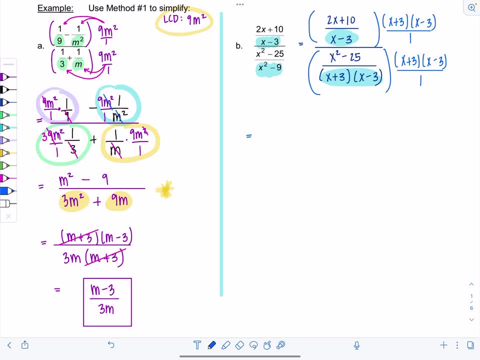 Okay, now let's look here at the numerator. When we distribute, x minus 3 will cancel out, But I still have that 2x plus 10 and x plus 3.. So I'm going to write that out here: 2x plus 10, x plus 3.. 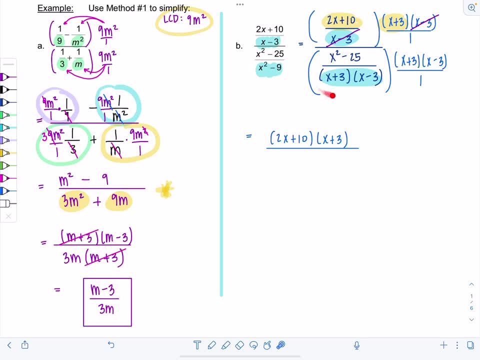 All right, now let's turn our attention to the denominator here. Both the x plus 3 and x minus 3 will cancel out, So all I have to do is write that out here, And then I'm going to write that out here. 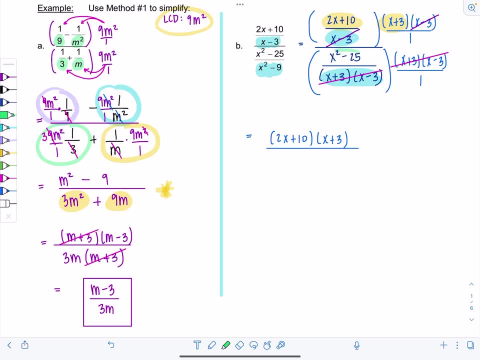 All I have left is x squared minus 25.. So that's going to go in the denominator. Okay, perfect. Now remember you are not allowed to do any canceling until the numerator and denominator are both fully factored. So not everything is factored. 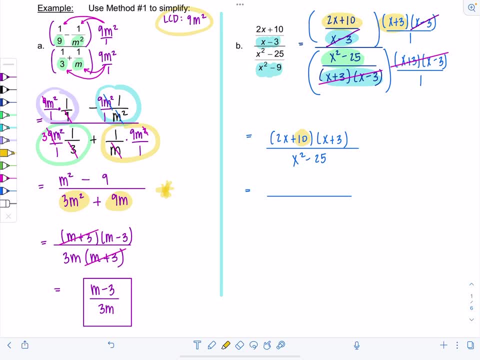 Let's go ahead, take care of that. I'm going to turn my attention to this: 2x plus 10.. I can take a 2 out right, So we have 2 times x plus 5 times x plus 3.. 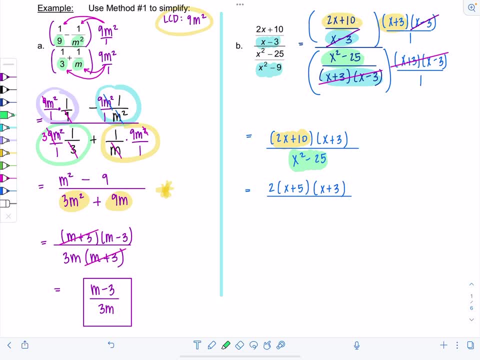 And then what about this x squared minus 25? How do we factor that? It's a difference of squares? so that's going to factor into x plus 5 times x minus 5.. Alright, perfect. And then, ooh, I noticed I can cancel out this x plus 5.. 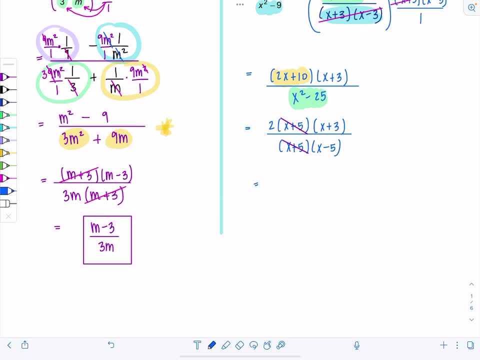 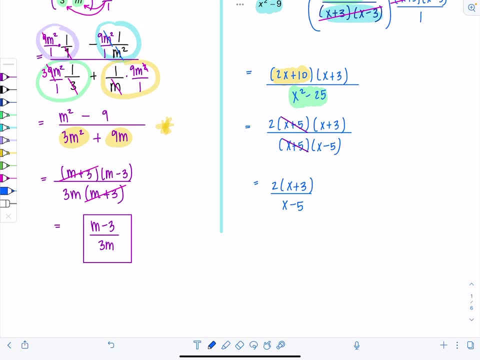 And then, final answer, we're left with 2 times x plus 3 over x minus 5.. You can stop there, or if you want to distribute the numerator, then it would be 2x plus 6 over x minus 5.. 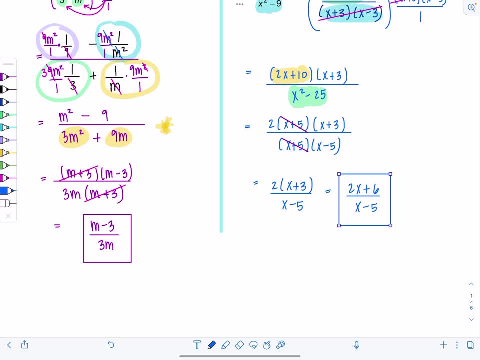 It doesn't really matter in this case. Okay, Very good. So that's the first method. I like using that most of the time, But on occasions another method is a little bit more advantageous to use. So let's look at what method 2 is. 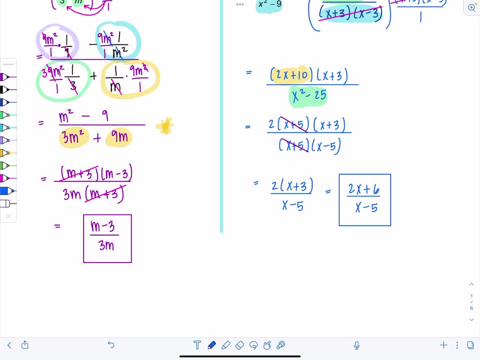 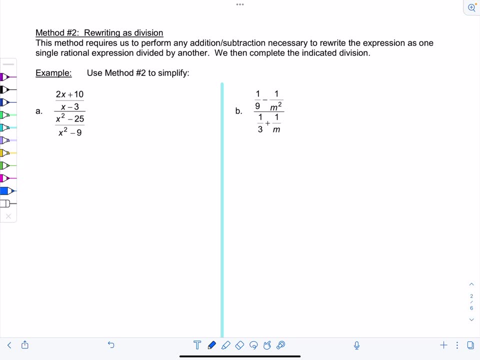 And you don't have to worry which one's method 1, which one's method 2.. Just know that there's two ways to do it. Who cares what number it's called? Okay, method 2 is rewriting as division. So this method requires us to perform any addition or subtraction necessary. 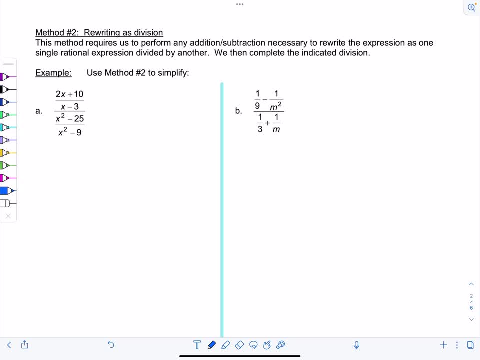 to rewrite the expression as 1, and if we have a single rational expression divided by another, we then complete the indicated division. So what does that mean? It means you're going to end up rewriting this fraction bar as the division sign, right. 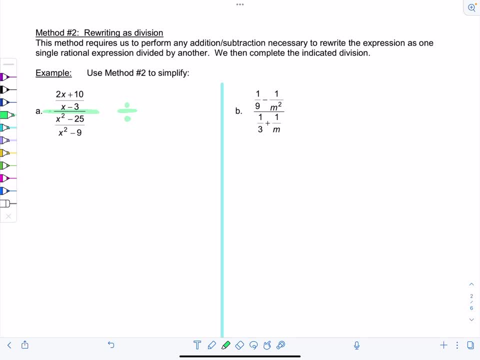 Because it means the same thing And you're going to divide the numerator by the denominator. It's just that before you get to that step, you have to make sure that your numerator is one term and your denominator is one term, In this case. you know what? 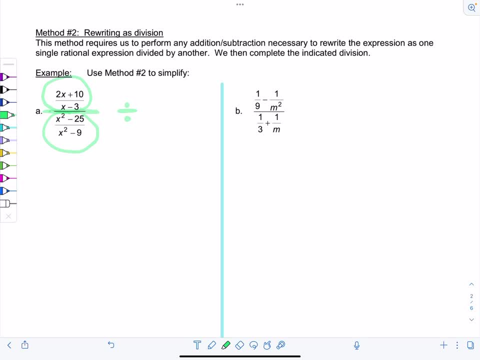 It is already, So we can just jump straight to that step. We kind of lucked out. So this is a nice example where this method might be easier than the first way we simplified. Okay, so we have here 2x plus 10 over x minus 3,. 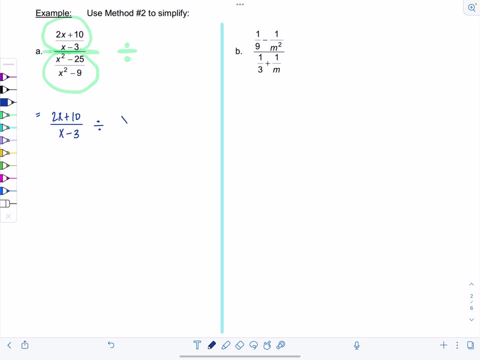 and then I'm going to write instead: divided by x squared minus 25 over x squared, So that's 2x squared minus 9.. Good, Okay, Then the next step. remember, when we're dividing two fractions, you want to change the division to multiplication. 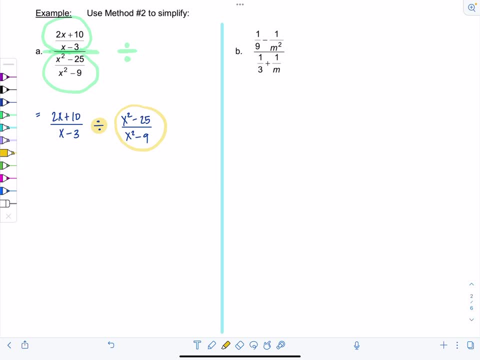 and then flip the second fraction, Multiply by the reciprocal. And while we're doing that, I'm going to factor everything too, Okay. So instead of writing 2x plus 10 in the numerator, I'm going to write 2 times x plus 5. 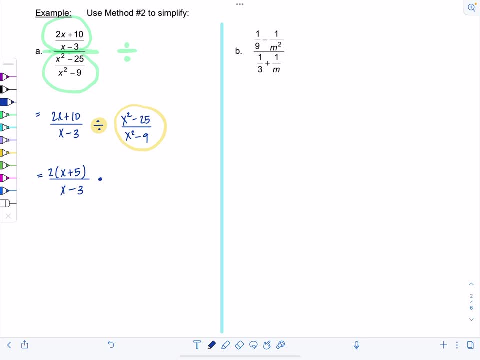 over x minus 3 times, and then we would have here x squared minus 9 in the numerator, but that's just x plus 3 times x minus 3.. And then we also have x squared minus 25 in the denominator, but that's just x plus 5 times x minus 5.. 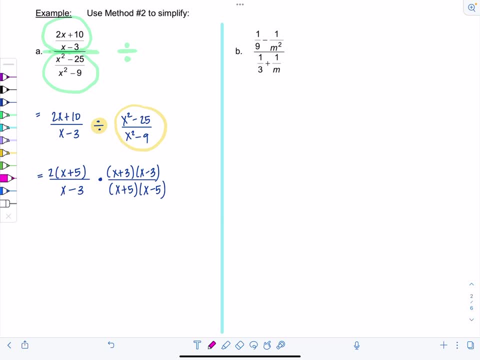 See how nice. Now everything is factored and we can go ahead and start canceling. Okay, So we're not canceling any common factors if they're on opposite sides of the fraction. So notice, here I can cancel out this x plus 5.. 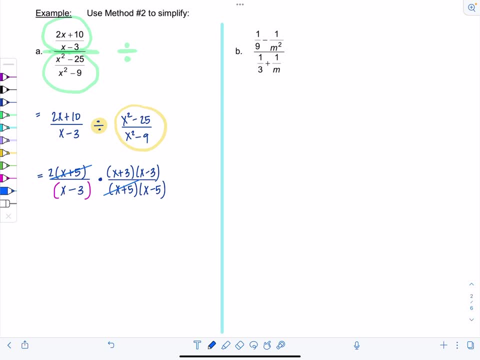 Even though they come from two different fractions. if one's in the top, one's in the bottom, they can cancel out And the x minus 3 can cancel out. But that's it, Okay, That's it. This x plus 3, that's a little family. 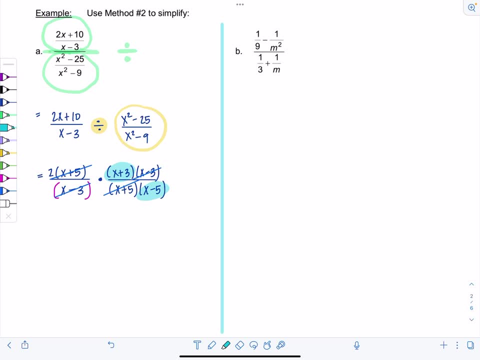 This x minus 5, that's a little family. Don't go in there and start doing something weird like canceling these x's. No, no, no, Then you'd be a homewrecker. you know We can't have that. 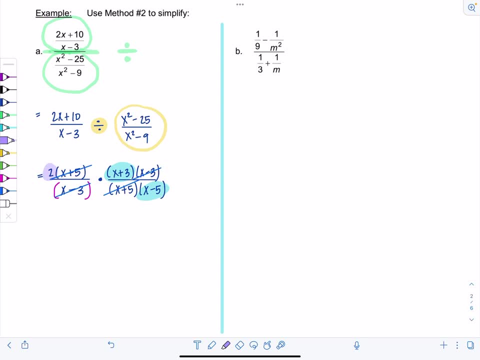 We cannot have that. So here we've got the 2 left over, x plus 3 left over and x minus 5 left over, So we have 2 times x plus 3 over x minus 5.. And notice same exact result. 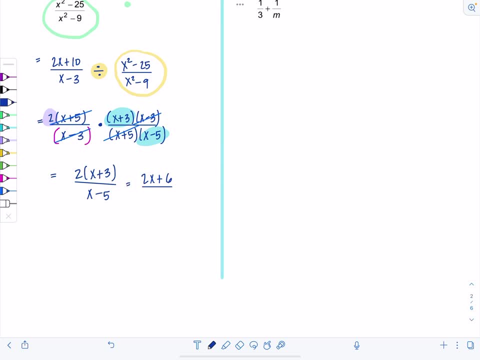 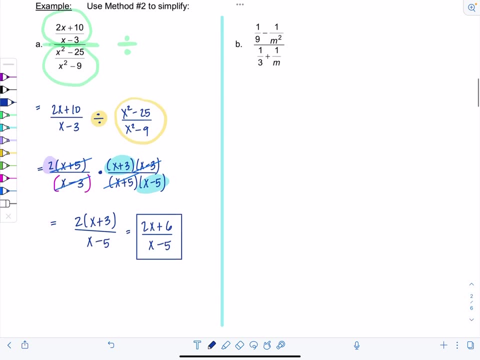 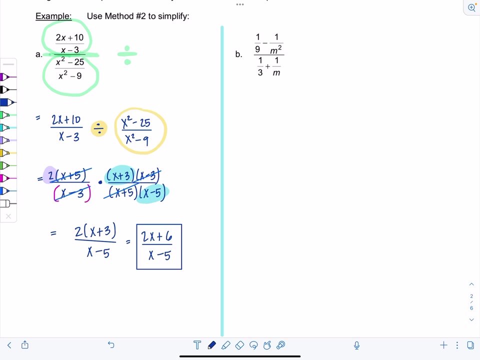 as when we did this problem just a minute ago using the other method. Which way, would you say, is easier? I don't know. They were both probably the same, huh, Okay, Next example. this one's going to take a little more work. 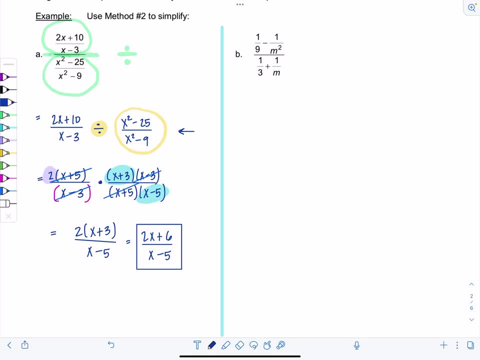 We can't jump straight to this step yet, because you see how we have two terms in the numerator and we have two terms in the denominator. We have to add those together or subtract them first. Okay, So let me rewrite everything nice and spaced out. 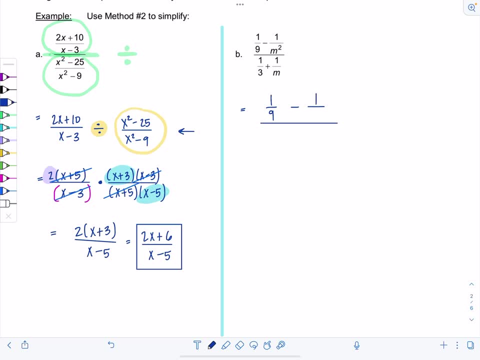 So we've got 1 9th minus 1 over m squared. So what's the common denominator? just for these two terms, Not the whole expression, Just in the numerator. what's the common denominator? It's just 9 m squared, right? 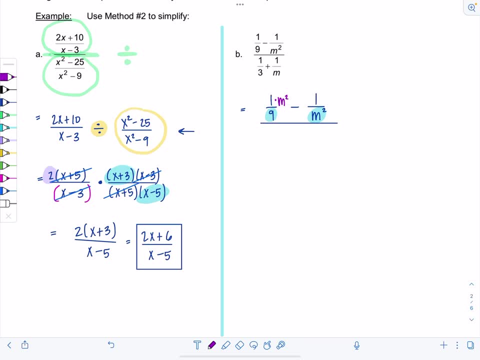 Okay, So I would need to, in order to get a common denominator, multiply this first fraction by m squared over m squared, And the second one by 9 over 9.. Lovely, Now let's look at the denominator. We have 1 3rd plus 1 over m. 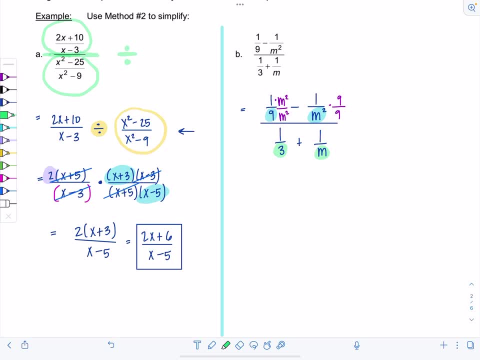 What's the common denominator? just for these two terms down here, It's 3 m, right? So we'll multiply this first fraction by m over m and the second one by 3 over 3.. All right, So let's see what we have here. 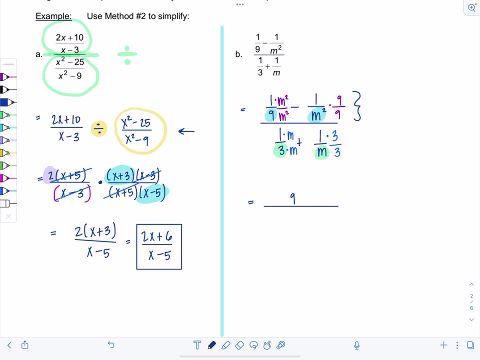 Remember, in the numerator my common denominator ends up being 9 m squared, And then I have 1 times m squared right here. So that's just going to give me m squared minus 1 times 9,, which is 9.. 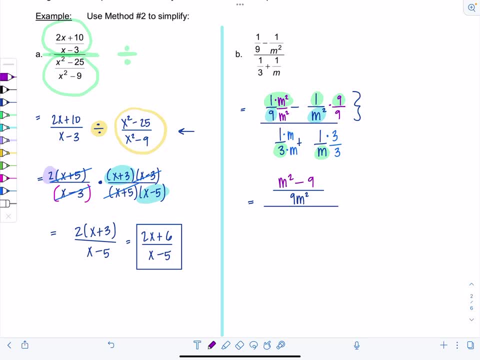 So we've got m squared minus 9 over 9 m squared in the numerator And then in the denominator. our common denominator was 3 m, And then check it out: We've just got 1 times m, which is m. 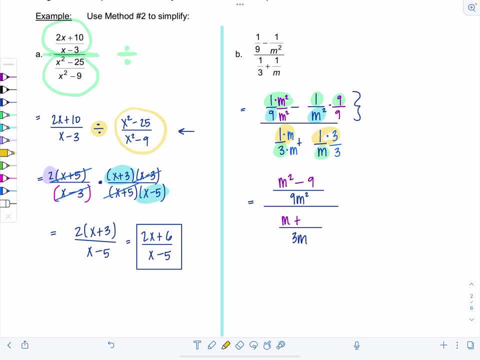 plus 1 times 3, which is just 3.. Okay, Lovely. Now we're basically at the same step that we were at when we got problem A given to us. So here's one term, One term, Yeah, And we can rewrite this fraction bar. 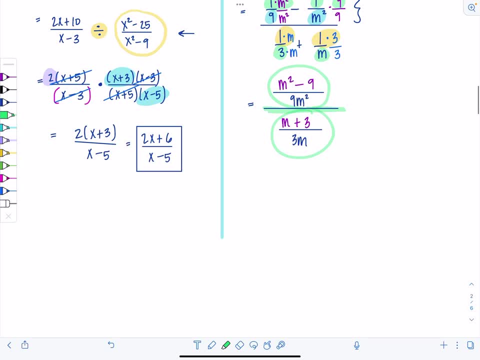 as division instead. So let's go ahead and do that. We have here m squared minus 9 over 9 m squared divided by m plus 3 over 3 m, And then from here you're just going to rewrite the division as multiplication. 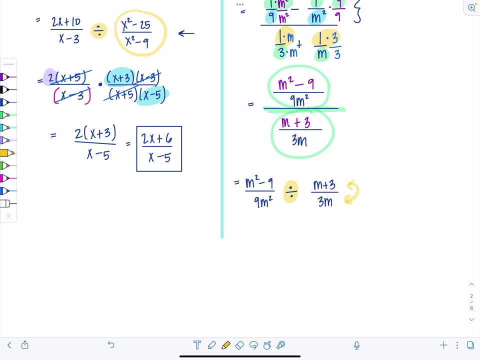 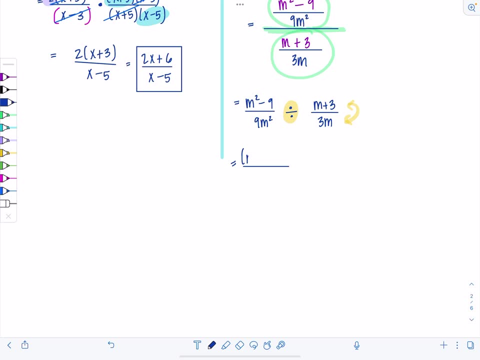 And then flip the second fraction And at the same time I'm going to factor everything. So m squared minus 9,. that factors into m plus 3, m minus 3,, 9 m squared. can't do anything with that. 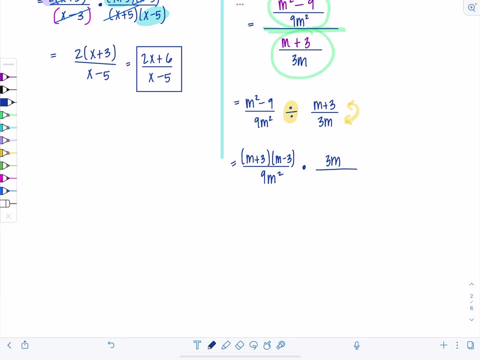 times 3 m over m plus 3.. And I'm going to put some parentheses around the m plus 3, just to remind me that's a factor. that's a little family If I do any canceling. they got to stay together. 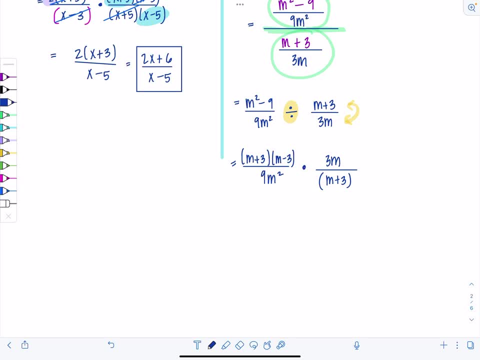 Anything we can cancel. This is always my favorite part, So satisfying m plus 3, bam bam, 3 m gone. With the 9 m squared it's going to become just 3 m, right, Very good. 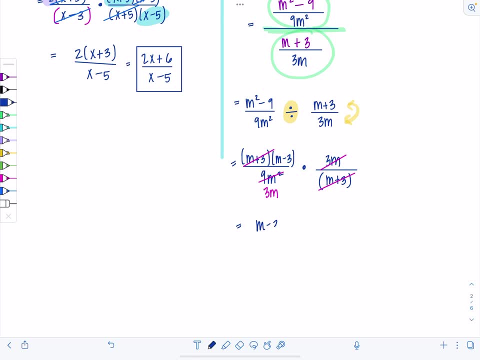 So now we're left with m minus 3, minus 3, over 3 m. Okay, And you can check. this is the same result that we got when we used the other method. Honestly, I like method one better for problems like this. 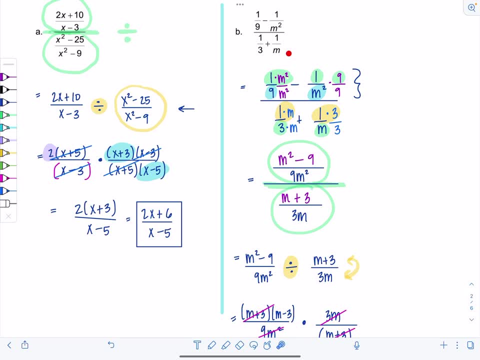 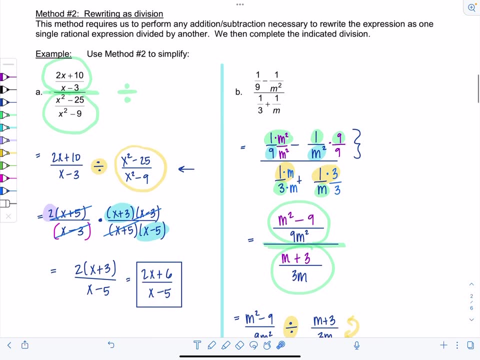 because I feel like it's a lot of extra work when you have to go ahead, get the common denominator first and then divide and do all this flipping. Okay, This method is nicer when the numerator is already one term, one fraction. 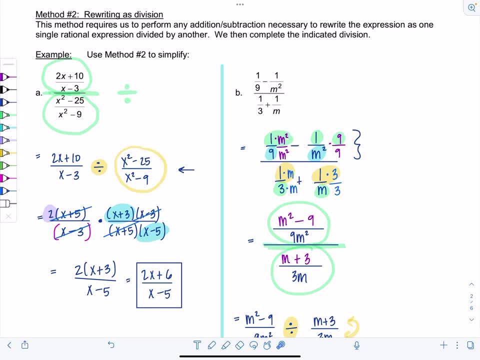 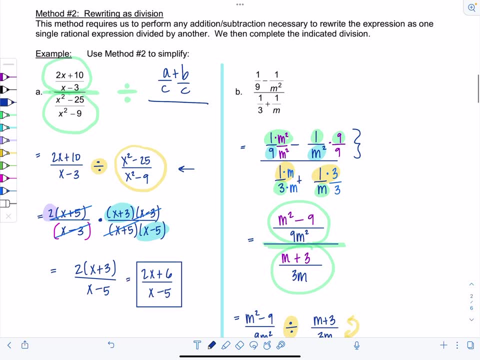 and the denominator is already one term, one fraction. If I see that you, like I, have a plus b like this over and there's more stuff than already, I don't want to do this method. It's just going to get too messy. 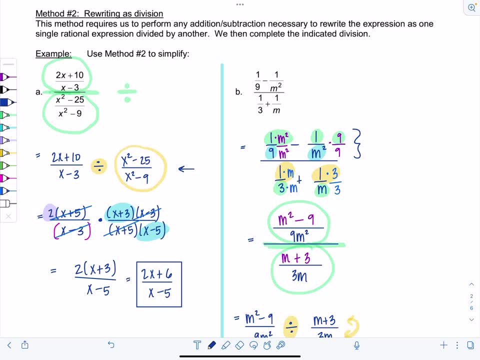 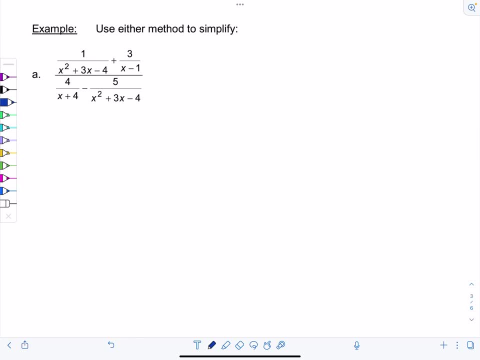 That's my personal taste. okay, You live your life, Just get them right. So here's another example. It says: use either method to simplify. Honestly, I'm just going to do the first method because I'm noticing there's two firsts. 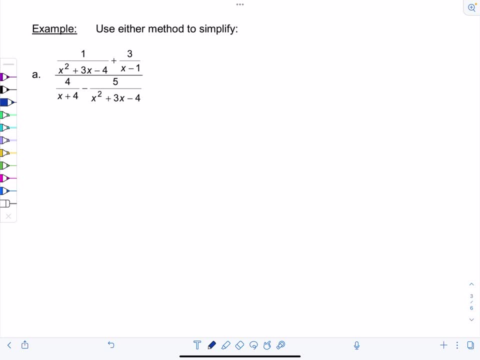 and then there's two firsts. I'm noticing there's two fractions in the numerator, two fractions in the denominator. I don't want to deal with adding and subtracting them first and then dividing Just sounds like a pain. I'd rather just be. 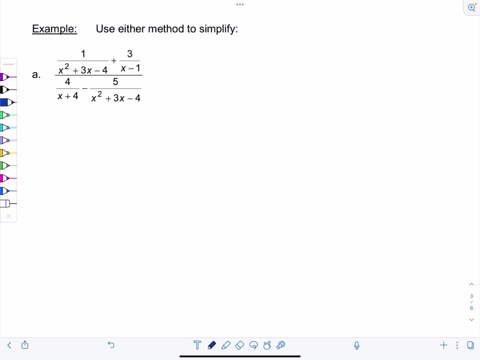 fraction-free. hit everything with the LCD from the get-go. Now, in order to identify the LCD, I have to factor all the denominators, So let's go ahead and do that first. So we've got 1 over, let's factor. 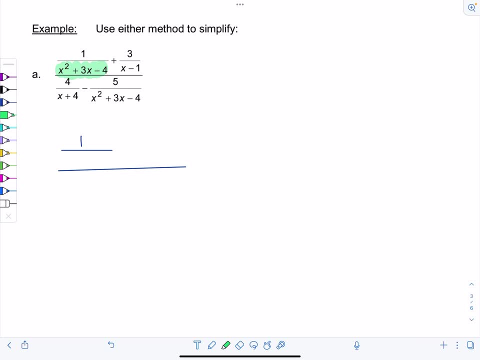 x squared plus 3x minus 4.. So how does this work? How does that factor? Very good, x plus 4 times x minus 1.. If you need a review on factoring, I'll link some videos here and in the description box. 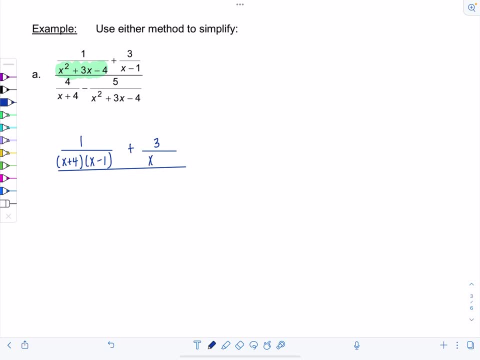 Plus, then we have 3 over x minus 1.. If you want to put parentheses around it, cool. And then in the denominator 4 over x plus 4, that's done. minus 5 over. now we have to factor again. 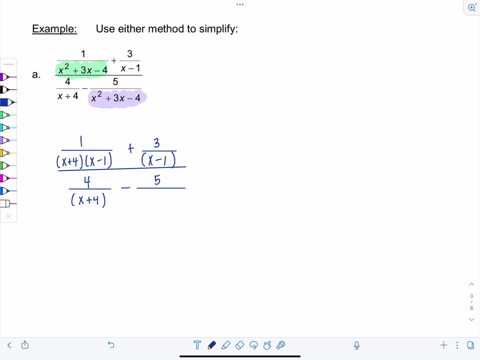 x squared plus 3x minus 4.. But we just factored it, So no big deal: x plus 4, x minus 1.. Okay so you guys tell me what is the LCD of all the minor denominators? What are the minor? 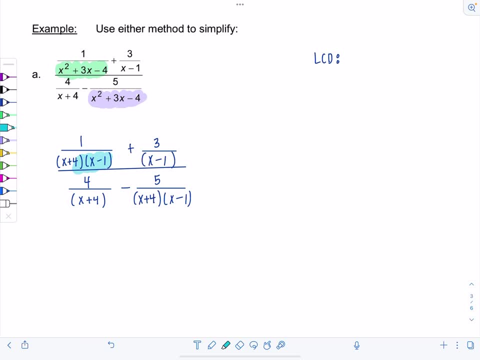 denominators. We've got four of them Here, here, here and here. So the LCD for these four guys is minus 5 over x plus 4 times x minus 1.. So I'm going to multiply everybody in the numerator. 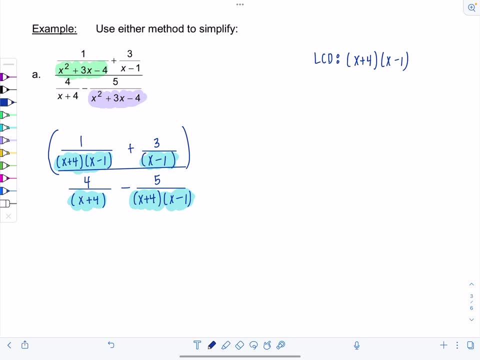 by x plus 4 times x minus 1, and everyone in the denominator by the same thing. If you want to remind yourself that each of these is over 1, go for it. Okay, how are we doing so far? So what are we? 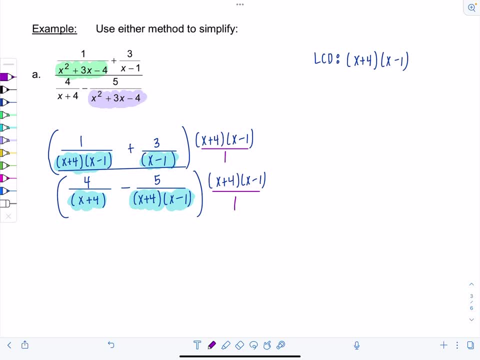 doing so far. Now, at this step, remember you're going to have to distribute as you multiply out the LCD to the numerator and denominator. When you get more comfortable, you could probably distribute and cancel in your head. I'm assuming you're not. 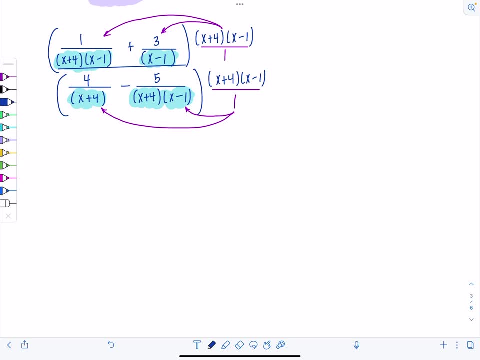 there yet. so I'm going to write the LCD next to each of the terms and go through this again. So we have 1 over x plus 4 times x minus 1, and then that's going to get multiplied by x plus 4. 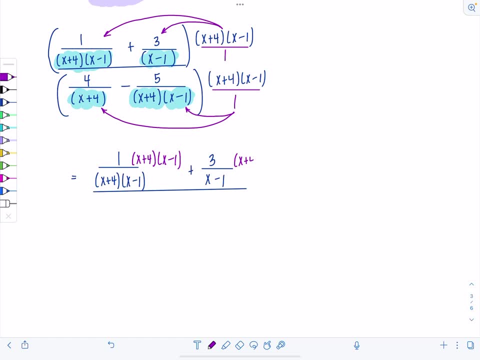 times x minus 1 plus 3 over x minus 1.. That gets multiplied by x plus 4. that gets multiplied by x plus 4 times x minus 1.. Remember that LCD always goes in the numerators when you're distributing minus. 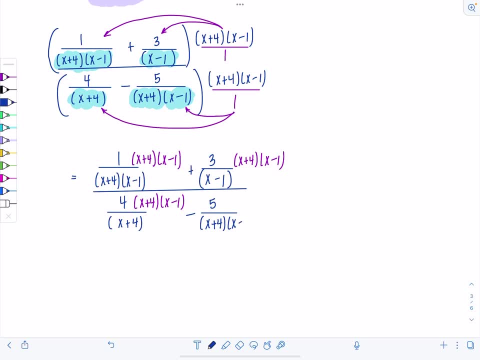 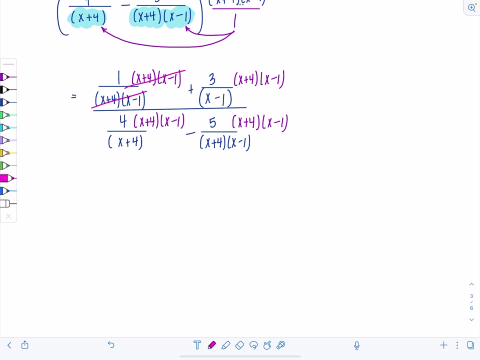 5 over x plus 4 times x minus 1, and that's going to get multiplied by x plus 4 times x plus 4.. Now my favorite part: cancel party time. So bam, bam those. completely cancel out x plus. 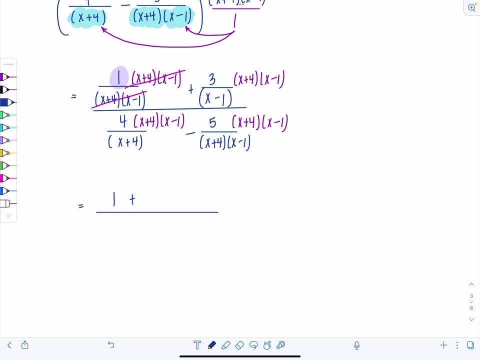 4 and x minus 1.. So all that we're going to be left with for that first term in the numerator is a 1.. So we have 4 times x minus 1 left minus x plus 4 and x minus. 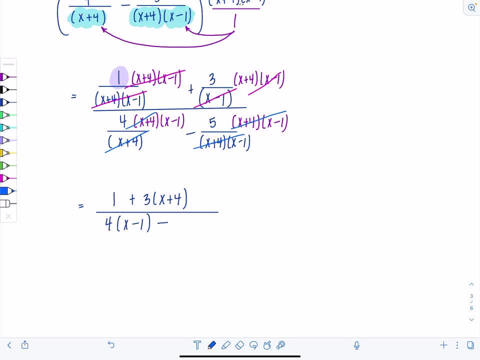 1, both cancel out. We just have 5.. Okay, how are we doing? so far? The worst is over. I promise Now no canceling can occur, because the numerator and denominators are not fully factored, It's only. 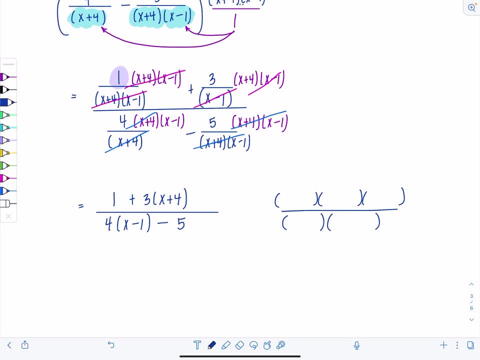 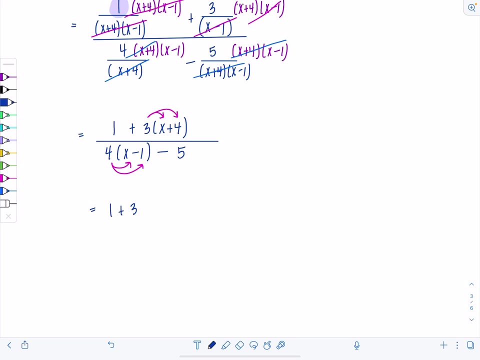 cancel time. when you have a C of parentheses like this, you know, then you can start canceling. But as soon as you have like parentheses, parentheses plus something, it's not cancel time, So don't throw that in the numerator. 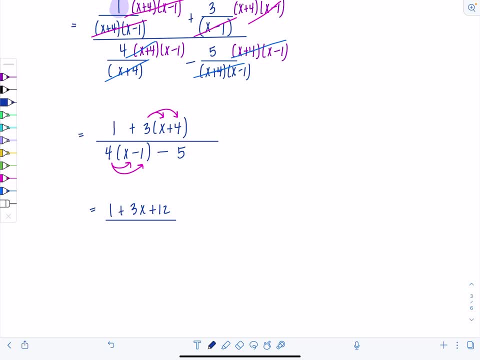 So we have 1 plus 3x plus 12 in the numerator over 4x minus 4 minus 5.. So let's see in the numerator 1 plus 12, that's 13. So we have. 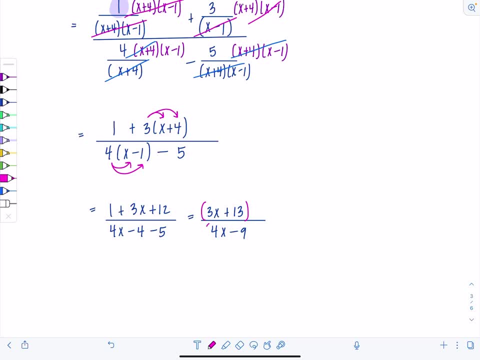 3x minus 4x plus 6x plus 5x plus 3x plus 2x minus 4x plus 6x plus 4x plus 6x plus 1x plus 9x plus 23x. 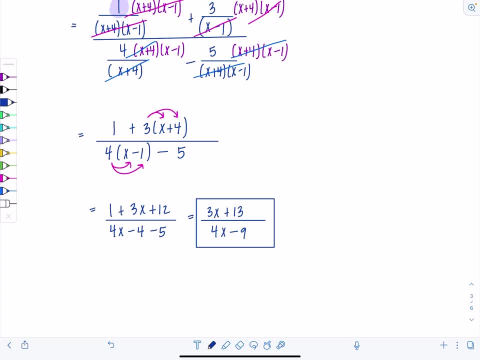 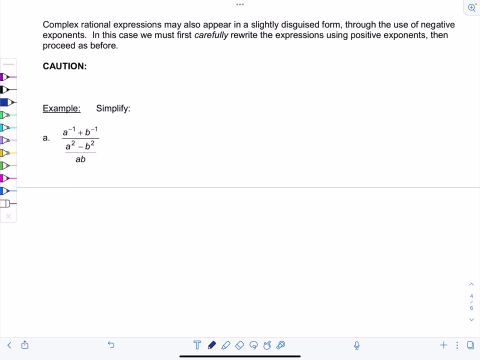 plus 7x plus 13.. 20, little more spicy. Complex rational expressions may also appear in a slightly disguised form through the use of negative exponents. In this case, we must first carefully rewrite the expressions using positive exponents and then proceed as before. And as a note of caution, 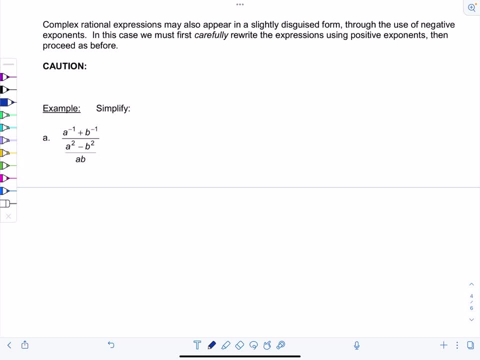 I want you guys to understand how negative exponents work. So if you have 3x to the negative first, that negative one exponent is only applied to the x because it's just touching the x, That's it. So you would rewrite this as 3 over x. But if you have 3x in parentheses, like this, raised to: 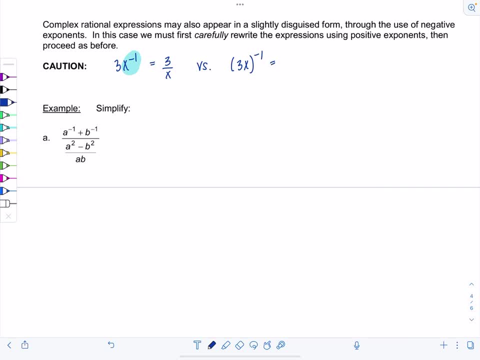 the negative first. then you would rewrite that as 1 over 3x, because the parentheses means that negative one Exponent applies to both the 3 and the x. Do you see the difference? Okay, good, So we're going to. 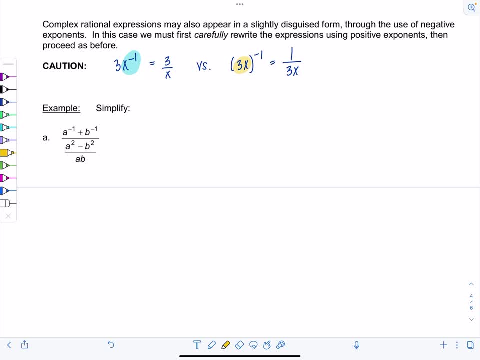 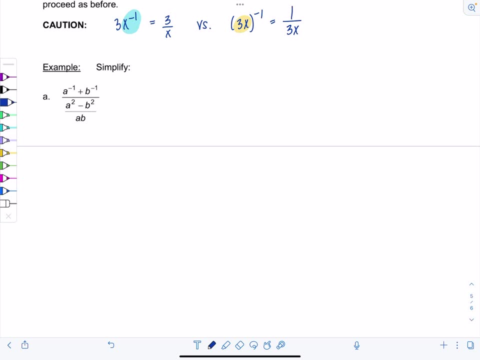 have to do that now. in the next example, where we simplify, We have a to the negative first plus b to the negative first, over a squared minus b squared over ab. So first things first, let's rewrite a to the negative first and b to the negative first as 1 over a plus 1 over b. 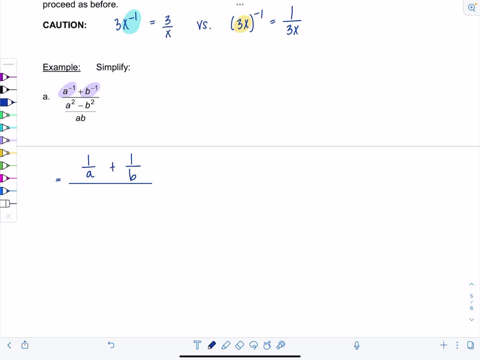 Good, Okay, and then in the denominator we have a squared minus b squared over ab. Now I'm going to use method one first to simplify. So in that case we're going to multiply by the LCD of all the minor denominators. So look here at the denominators. We've got an a, a b and an ab. So what's the LCD? for those three denominators. We've got an a, a, b and an ab. So what's the LCD for those three denominators? We've got an a, a, b and an ab. So what's the LCD for those three denominators? 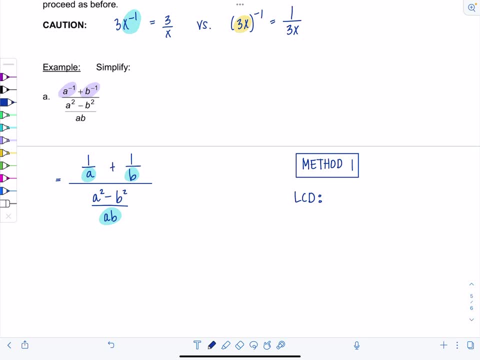 That's right, it's ab. So that's what I'm going to multiply everything by in this expression. I'm just going to already distribute it like this: ab, ab, ab, Okay, And then now we can cancel and clean up. So let's see here. 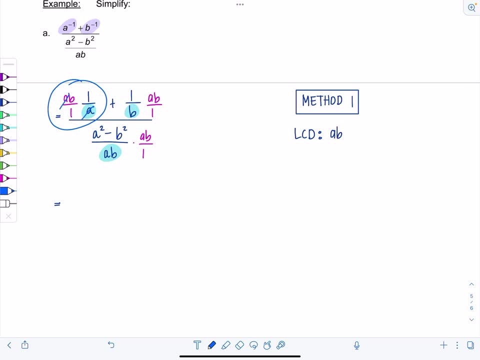 In this first term, a cancels out, So I'm just left with a, b, cool plus. and then let's look over here: b is going to cancel out, so we're just left with a. and then now please turn your attention to the denominator. 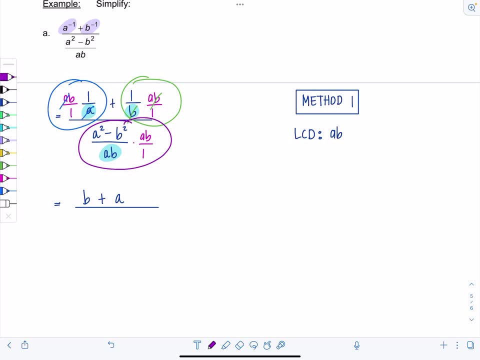 and I notice, oh, a, b cancels out, so I just have a squared minus b squared. okay, perfect. now let's see here. are we on the right track. do we have any fractions left in the numerator or denominator? no, we don't, so it looks like things are headed in the right. 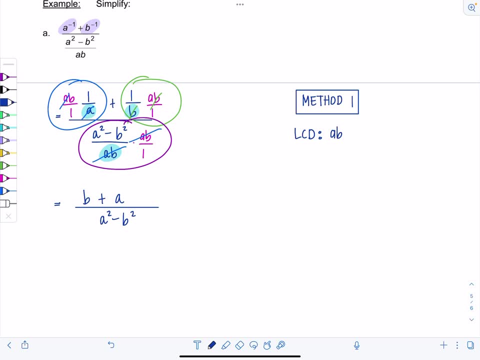 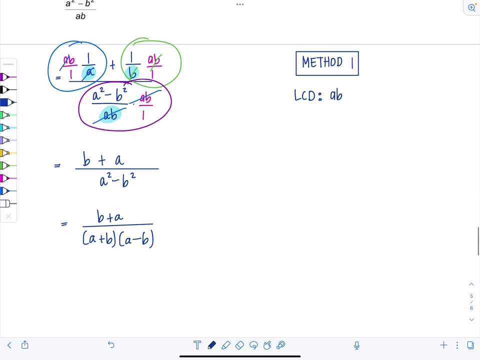 direction. now from here. I want to see if I can factor the numerator and denominator more and then maybe simplify after canceling numerator is done: b plus a. okay, denominator: a squared minus b squared. you can factor that into a plus b, times a minus b and keep in mind, since addition is commutative, adding the order doesn't matter: a plus b and b. 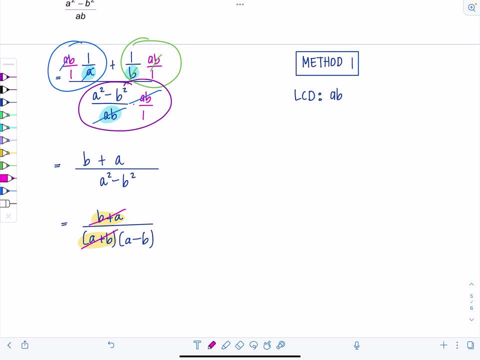 plus a are the same factors. these cancel out. don't forget, though, you still have that one right in the numerator when everything cancels out from upstairs, so your final answer is going to be one over a minus b, so I can do this over a minus d, and that the first two lines that we're going to do is going to: 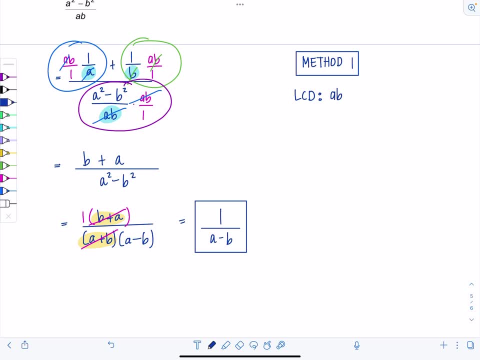 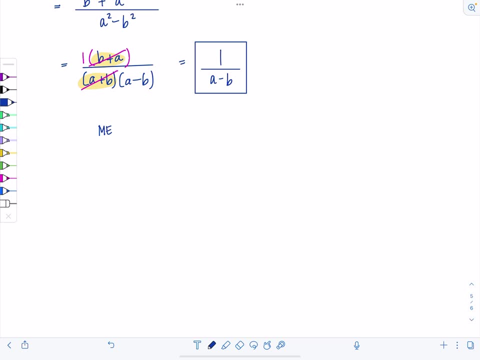 be one over a minus b. okay, how was that not the worst one we've done? huh, I think the previous example was a little more tricky. now how about trying this with method two, just so you can compare. so let's try it with method two. and originally I'm just going to jump to after we rewrote this with the negative exponents in the denominator. okay, so here I'm going to go. had an. 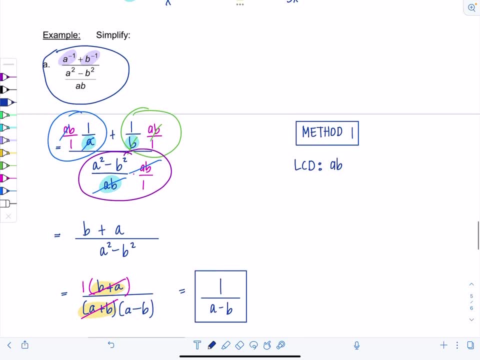 but is this Lakota? so we're бойed in several times with that. so вкусenke is not a leavel, a Grammy. I don't know what the problem with that sentence left I'm. we rewrote this with the negative exponents in the denominator. okay, So method two. 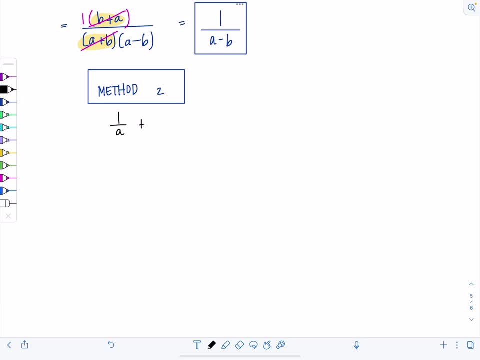 if we have one over a plus one over b, over a squared, minus b squared over ab. So method two basically says: if there's addition or subtraction in the numerator or denominator, you do that first, and then you rewrite this division, this fraction bar as the division sign. after you do that. 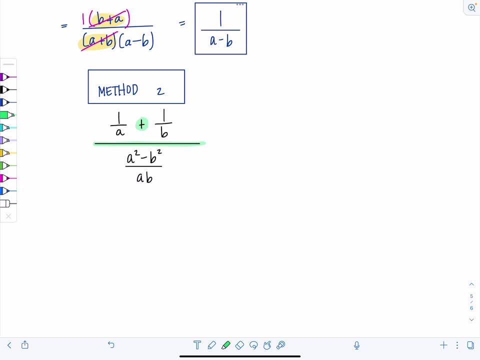 Okay, so let's look here at the numerator. If I want to add these two terms together, what would my common denominator be? It would be ab right. So I'm going to multiply this first term here by b over b and the second one by a over a. Very good, And then the denominator. 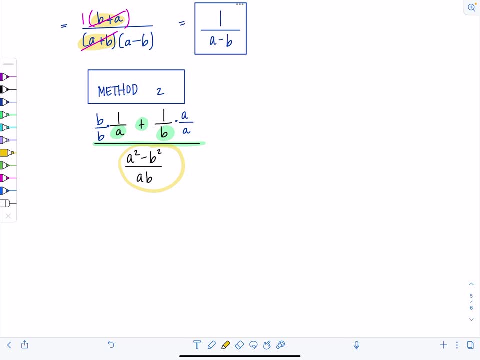 I don't have to do anything with, because you see how it's already one, one fraction, it's one term. So in this method you just leave that alone. It's happy minding its own business over there. And so in the numerator I'm going to have b times one, So that's just b. 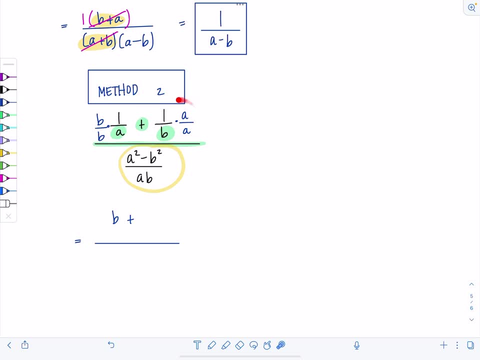 That's for my hair, Plus a times one which is just a over ab, And then this is over a squared minus b squared Over ab. Very good, Now we rewrite the fraction bar as division. So in the next step I'm going to. 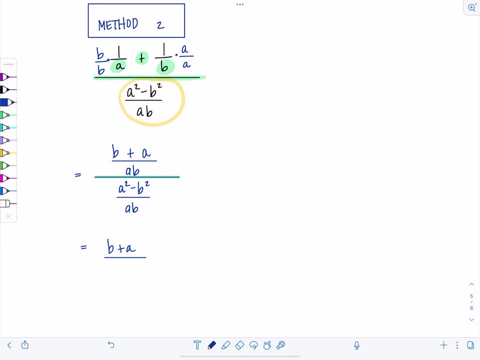 have b plus a over ab, divided by a squared minus b squared over ab. Good, And then next thing we need to do: change this to multiplication. flip the second fraction, leave the first one alone, So it's b plus a over ab times. 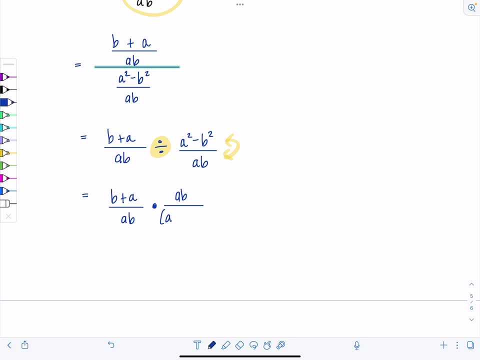 and then we have ab over. are you guys cool if I factor that a squared minus b, squared a plus b, a minus b, Yeah Lovely, And then right away I can cancel the a plus b with b plus a, and then I can also cancel ab with ab. So 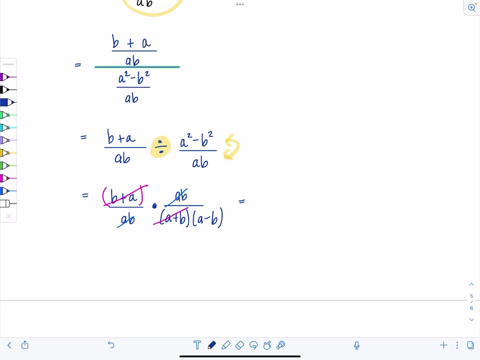 we're all done now. Since everything canceled in the numerator, I have a one. Don't forget that There's always a one left over when everything cancels somewhere- And then a minus b in the denominator. Very good, Very good. When you get comfortable, you might notice at this step, right. 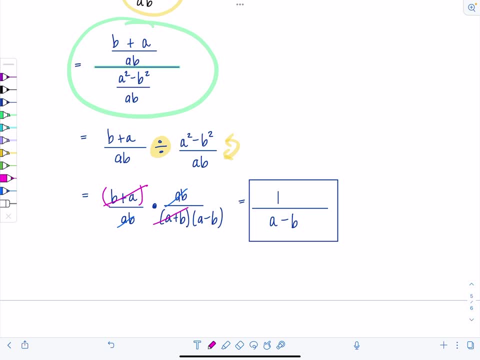 here. when you get semi-professional, you see how these denominators were the same. You can just cancel them because they end up canceling. So when you get comfortable, you might notice at this canceling right here at this step. if you want to skip all this, I'm cool with that. Maybe your. 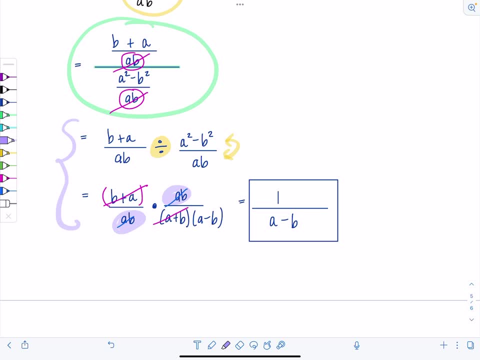 teacher won't be, though, so run it by them first, Okay. last example: I want you guys to pause the video before we keep going and see if you can rewrite this expression without negative exponents. first, okay, and then check in before you try to clean it up. So pause the video and then check back. 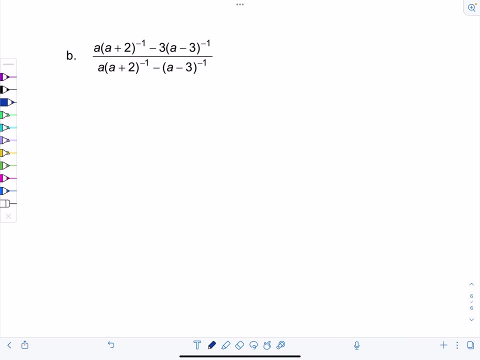 Okay, so this one's a little bit tricky. Notice that this a and this negative three are not in parentheses, so they're not going to get flipped to the denominator, since this negative one exponent does not apply to them. So the first term: we're going to rewrite it as a over a plus two, Do you? 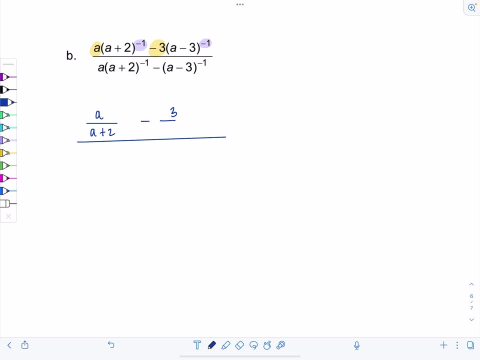 see that Minus three over a minus three, And then we're going to rewrite it as a over a plus two, And then in the denominator we're going to have again a over a plus two minus. And then, if I put a, 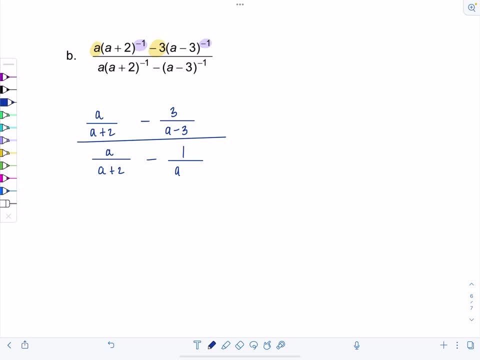 minus three in the denominator, I still have a one left over in that numerator, Lovely, I'm totally going to go with method one here. I don't feel like sitting there and doing this subtraction and then dividing and all that nonsense. Let's just cut to the chase. What is the LCD for all? 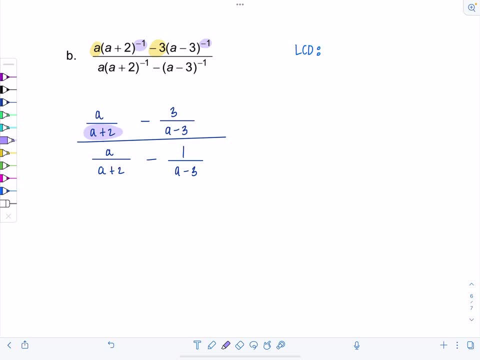 the minor denominators. So the LCD for a plus two, a minus three, and we got the same stuff going on downstairs. That's just going to be a plus two times a minus three. So let's multiply everything in the numerator and denominator by that And I'm just going to go ahead and write it. write that LCD. 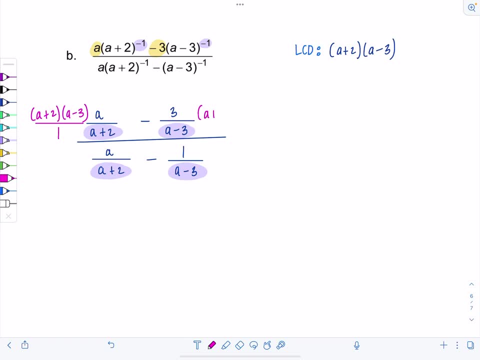 next to each term. Okay, I'm putting the over one just in case it's helpful, So you remember when we're canceling, where everything is And there's four terms. So everything's going to get multiplied by that LCD: A plus two, a minus three And, like I said, when you get more advanced you won't have to write it. 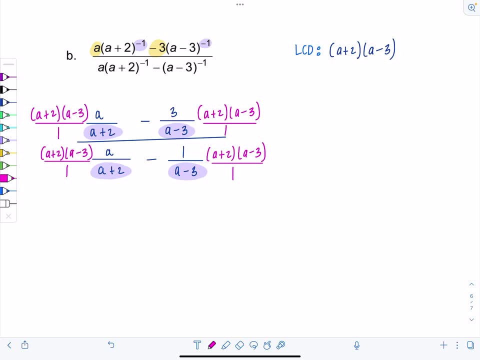 out next to each term. you'll be able to do it in your head. So it feels tedious right now, But with practice you'll get a lot more proficient at it and slick: Okay, Are we ready to cancel? I think so. I think so. So let's look at this first term. 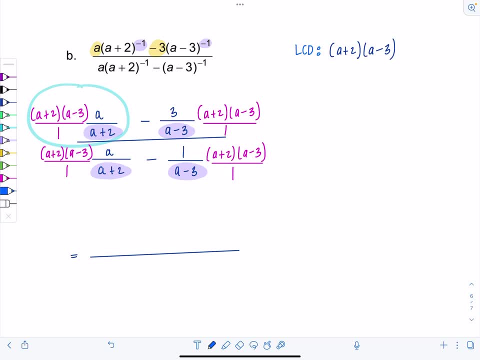 Here What's going to cancel the a plus two? So we're just left with a times a minus three, And then we have minus. okay, bring down that minus sign. And then what's left over here? Let's see. Let's see, A minus three cancels. So I have three times a plus two. Good, Now let's look. 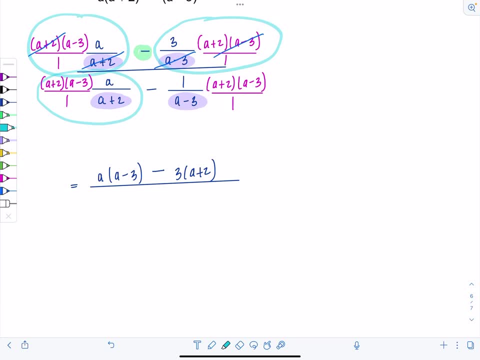 at the denominator here. What's going to cancel? A plus two, So I'm just left with now a times, a minus three. Bring down that subtraction sign, So we've got minus. And then last term a minus three is going to cancel And I just have a plus two. But please put parentheses on the a. 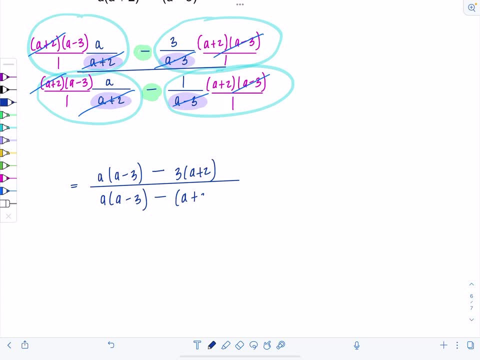 plus two Because that's going to cancel. So I'm just left with now a times a minus three And then I'm going to use that minus sign needs to distribute. Okay, This is a dangerous place for a lot of students. They get too excited and they start wanting to cancel. Oops. 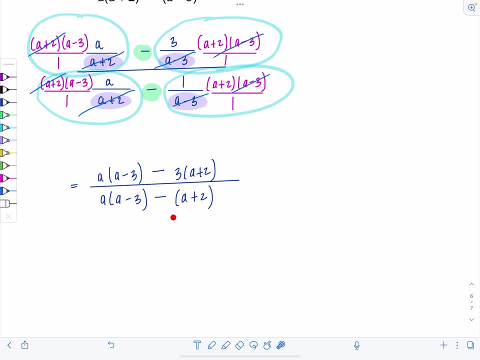 They start wanting to cancel out these terms that they see. But no, no, no, You're throwing your cancel party prematurely. The numerator is not completely factored. You see how we still see subtraction. Neither is the denominator. You can only cancel when everything is just a sea of. 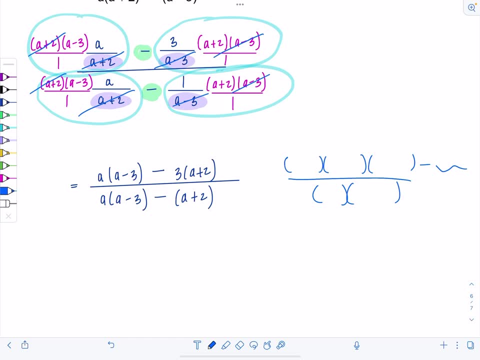 parentheses like this. So I'm just left with a minus three And then I'm going to use that minus the minute there's a minus something. Uh-uh, It's not cancel time. Everything's not fully factored, So you got to have some self-control. What does that mean for us? That means we're going to 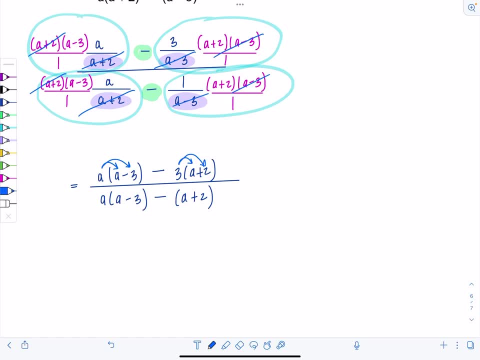 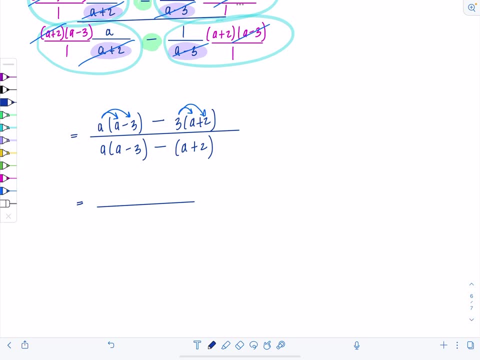 distribute, Oh yes, And then clean up and then see, maybe, after factoring completely, can we cancel. I know, I know. Okay, So we've got a squared minus three, a minus three, a minus six. Yeah, Good, good, good. 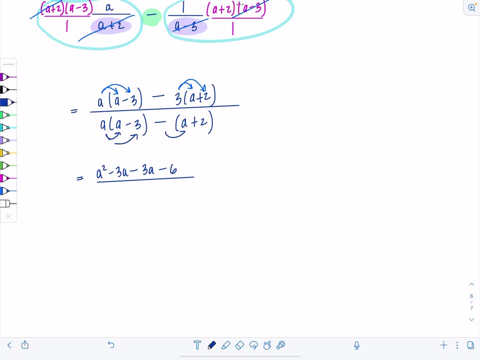 Over, And then same thing Distribute in the denominator. So we've got a squared minus three, a minus a minus two. And then let's combine our like terms. So we've got a squared minus six, a minus six, in the numerator, And then a squared minus four, a minus two, in the denominator.